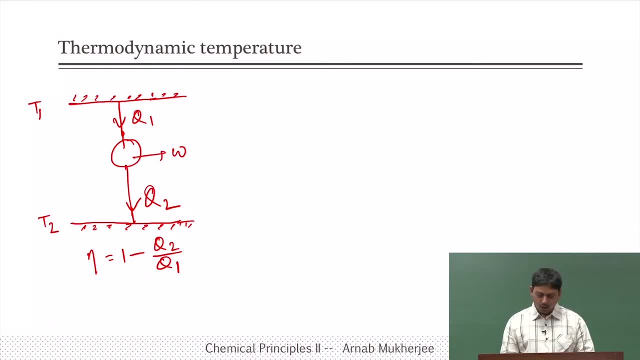 Q2 is heat that is thrown out to the low temperature. so you see, this efficiency, eta, which is 1 minus Q2 by Q1, depends on this two temperature, 2 temperatures, T1 and T2. right, so we can say that the efficiency is basically a function. 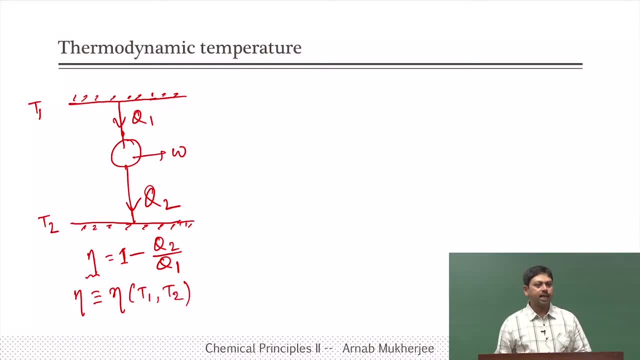 of 2 temperatures, T1 and T2, because nothing else is required to define the efficiency of a current engine apart from that, the heat taken in and heat, you know, thrown to 2 different temperature reservoirs. So we can call that this particular efficiency, some function. let us say Phi of T1 and T2. okay, 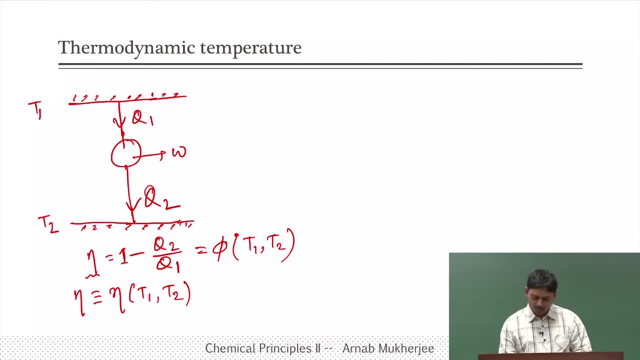 Now let us construct another engine, a combined system where 2 engine works simultaneously. heat Q1 is taken in from high temperature, some work is being done And Q3 is thrown to an intermediate temperature reservoir, T3, so T3 works as temperature reservoir, low temperature reservoir for the upper engine. let us call that A, and then same Q3 will be. 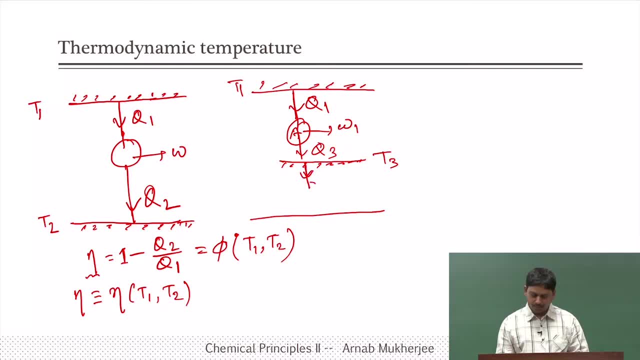 taken in by another engine called B, which does some other work, And finally, Q2 heat is thrown to the T3. T2 temperature reservoir. so what we have done is that we have replaced 1 engine by 2 engines and there is a temperature reservoir in between T1 and T2 temperature. okay, 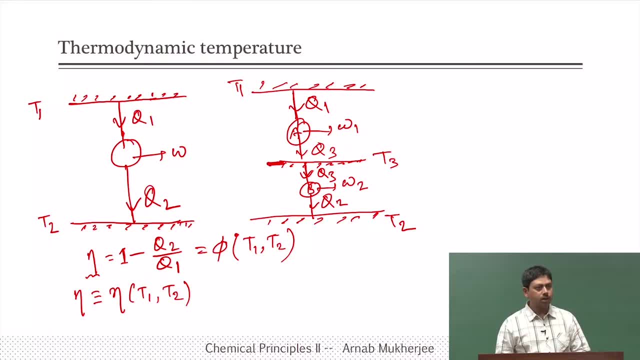 Since the heat cannot escape, it takes in and give the same amount of heat to the next engine. So now, this is a combined system. Now, if you calculate the efficiency of engine A, what you are going to get? 1 minus Q3 by Q1.. 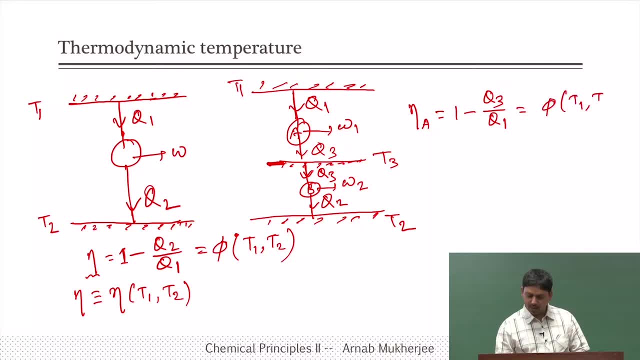 And this one. This is a function of T1 and T3, right. Similarly, eta B, which is the efficiency of the second engine, is 1 minus Q2 by Q3. Therefore you can say it is a function of T2. so we are writing like: first high and then. 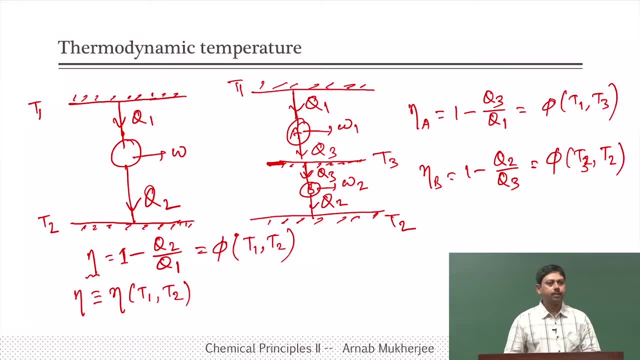 low. so T3 and T2, okay, Okay, Okay. So now you see, if I consider the final- you know initial and final- temperature differences, then efficiency of this engine let us call it C. So efficiency of engine C will be same as that of the combined efficiency of the right hand side engine. okay, 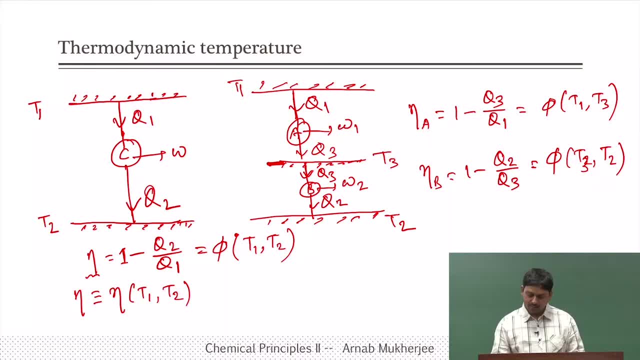 So now, if I rearrange a little bit here this particular equation, Let us say from here: if I rearrange a little bit, Then what I get is that Q2 by Q1 is equal to 1 minus phi, T1, T2. okay, 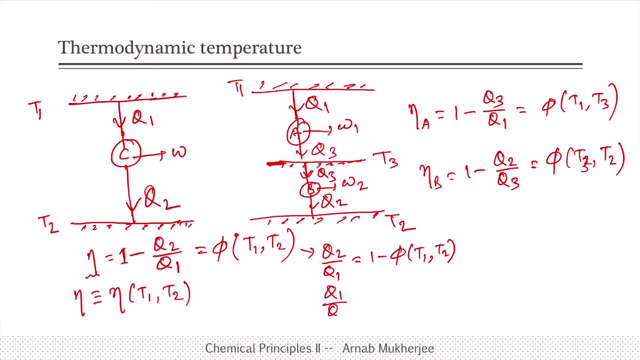 We can invert it and write Q1 by Q2.. So we are inverting, just to say that, heat input divided by heat output. Okay, Okay, Okay. So you can see that the efficiency of this engine is 1 minus phi, T1, T2, right. 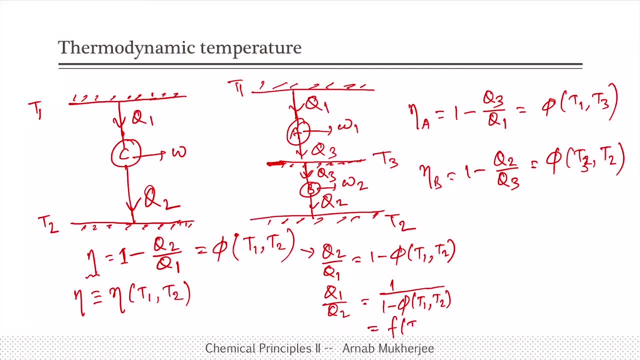 It is still a function of T1 and T2.. So let us call it F, T1, T2.. Now, finally, what we got For the engine C- we got Q1 by Q2 is equal to a function, that is a function of T1 and. 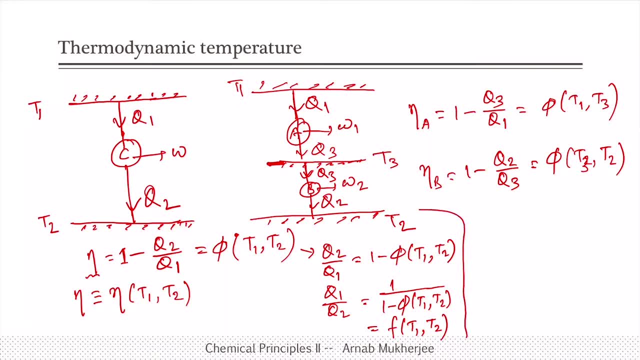 T2.. Okay, So we can write the same thing for above too. So from eta A we get Heat, input is Q1. by Q3 is a function of T1 and T3. and from Eta B, the engine B, what we get the input is Q3, output is Q2. we get F, T3, T2. now you see, one interesting thing happens. 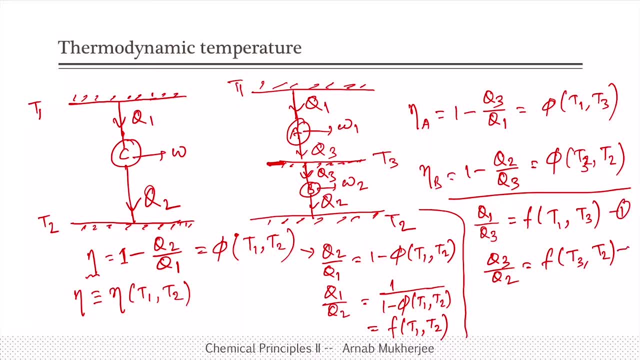 I can multiply equation 1 and equation 2. so if I multiply equation 1 and equation 2, what I am going to get- Q1 by Q3 into Q3 by Q2- is equal to F, T1, T3 multiplied by F, T3, T2 left. 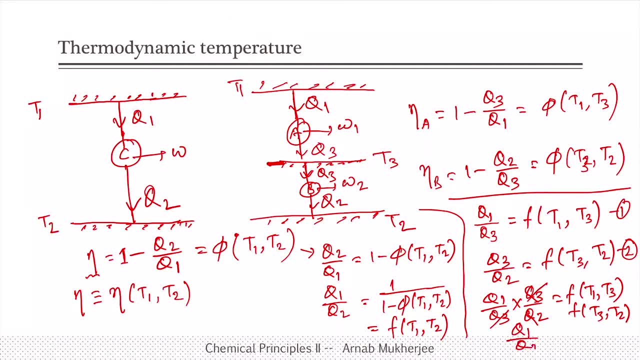 hand side cancels and gives us Q1 by Q2 is equal to product of Eta B, Two functions. okay. now this we get from here, let us call that equation 3, and we already have from this equation 4, Q1 by Q2.. 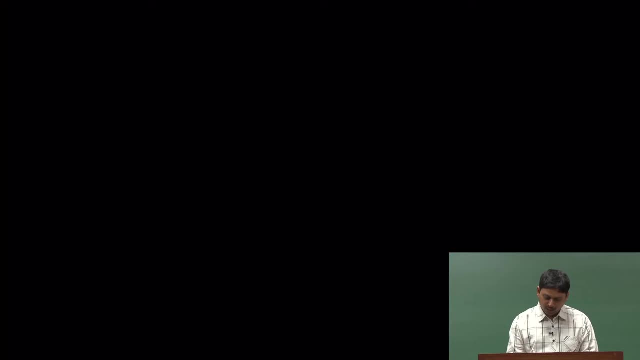 Now 4 and 3 we can equate. so what we have seen, that from engine C, from engine C we got Q1 by Q2.. Q1 by Q2 as a function of T1, T2, and from combined engine A and B we got Q1 by Q2 as 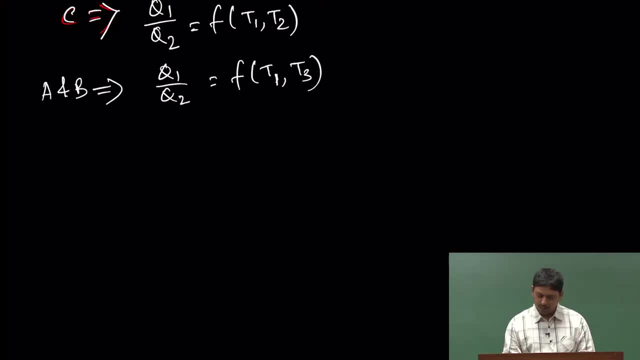 F, T1, T3 multiplied by T3, T2. okay, so equating these two, we get: T1, T2 is a product of T1, T3 as a function of F, T1, T3.. Okay, F, T3, T2. now you see, somehow this product of this functions is dropping out here, even though 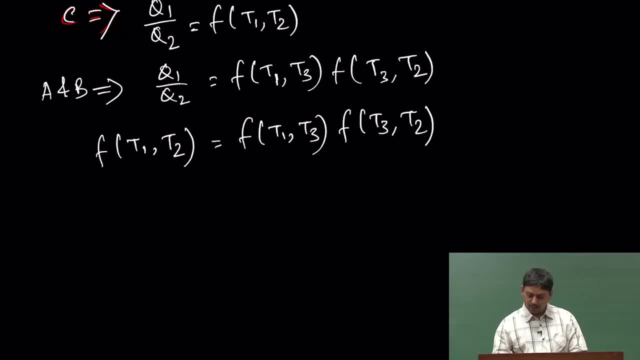 we have introduced a temperature and that is possible if this function- T1, T2 or any two temperature- is a ratio of function of these two temperature separately. Let us say: if I write in I can show you. so this can be a function of. so Psi T1 is a function. 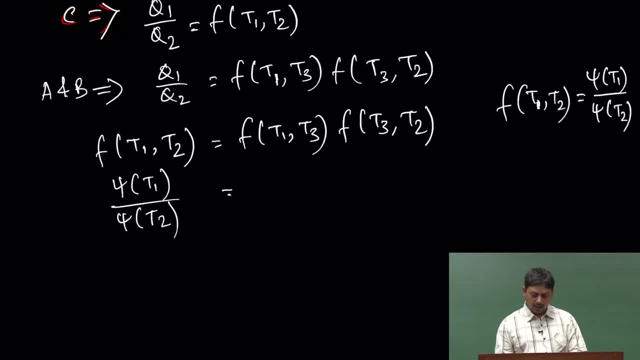 of T1 and this ratio is the overall function. we can write the same way, You see, if you write that the Psi T3 cancels out, so F is basically F, which is a function of two temperatures, is basically ratio of function of individual temperatures, right? 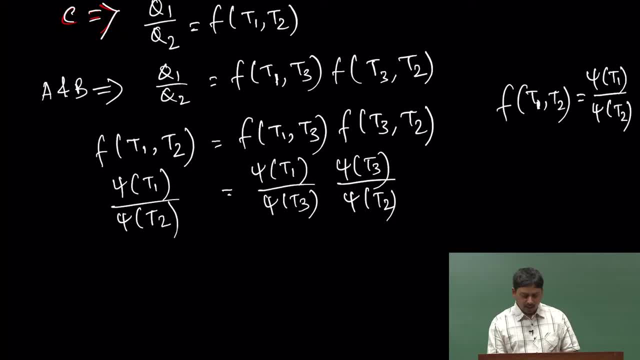 So now, what we learnt from here is that, and where did we get this? now, what is our F T1 T2.. Our F T1 T2 is nothing but Q1 by Q2, right, and we got F T1 T2 as Psi of T1 by Psi of T2. 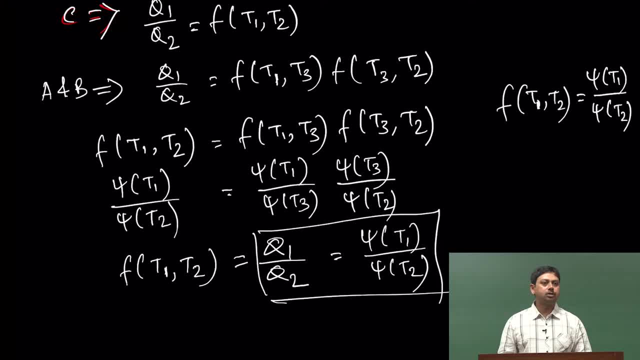 so this is the basic formulations of the thermodynamics temperature. So you see, it is not exactly a temperature, it is a function of temperature, some function of temperature. Now, Kelvin used a linear function. We can use some linear function which changes with T1, and if you use a linear function or 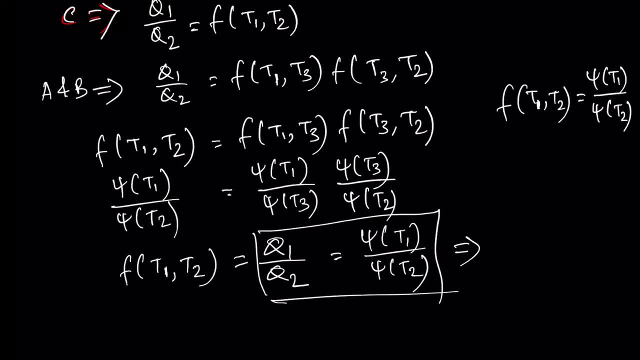 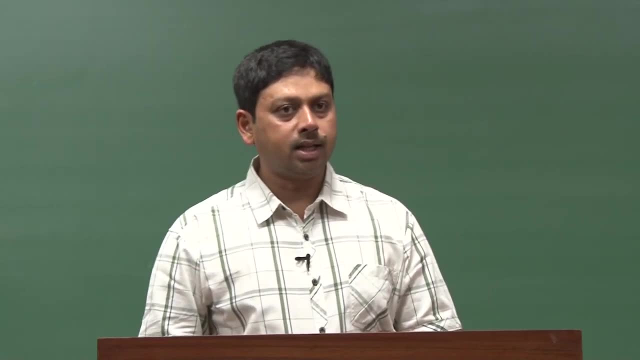 we can call this Psi T1 itself as T1, then we can say that the ratios of heat input output is related to the ratios of two thermodynamic temperatures. You only need one specific point in order to determine the other temperatures. so, for example, if you calculate Q1 and Q2 for a known temperature, 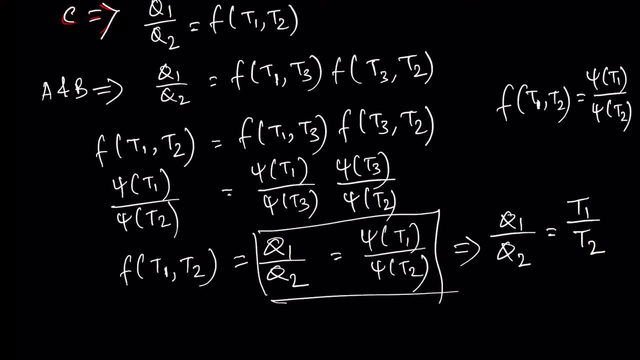 So this is the temperature of the thermodynamic temperature. So this is the temperature of the thermodynamic temperature. So this is the temperature of the thermodynamic temperature And the known temperature typically is taken to be the temperature of triple point of water, which is 273.16.. 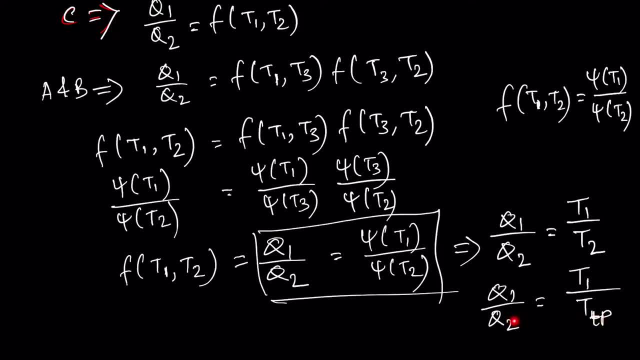 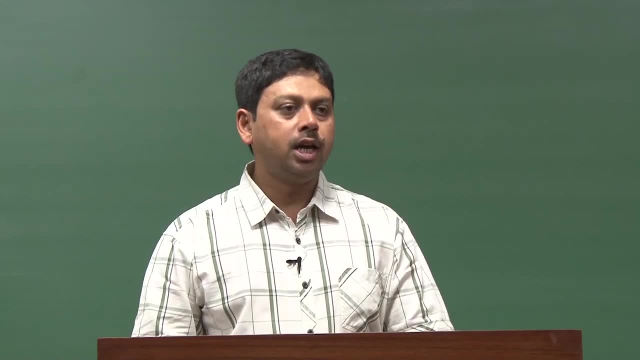 So this is T. triple point is known: Q1, Q2 will be measured and then you can get the value of T1.. So thus we can measure the temperature, given that we can calculate heat input and output. So in real experiment, especially below 1 Kelvin temperature, where the gas see other the temperature, 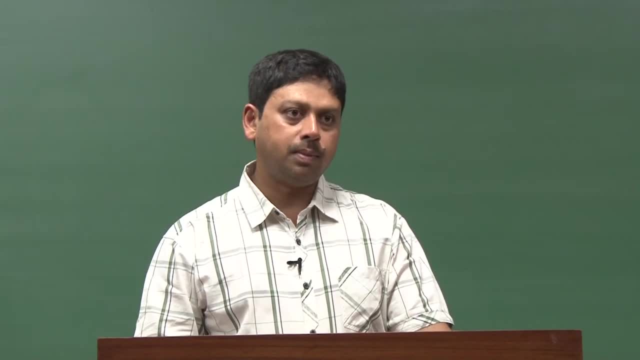 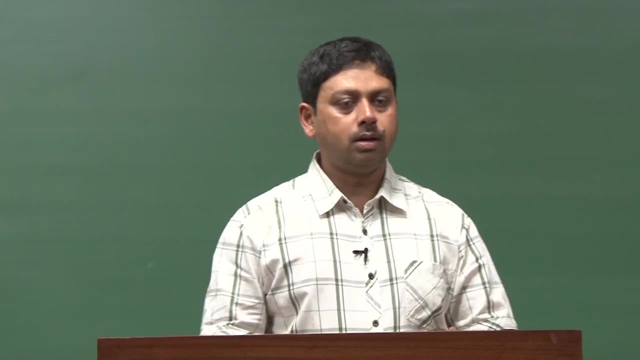 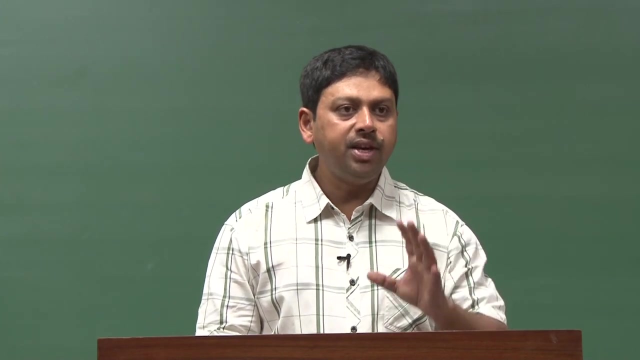 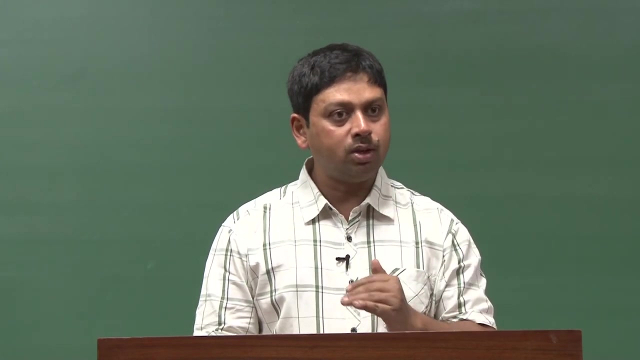 that we learn from. you know, zeroth law of thermodynamics is when we combine a property with the heat, So, for example, or with the temperature. for example, we say that how much is the value of PV when the pressure is very low and how much is the value of PV with respect to PV? 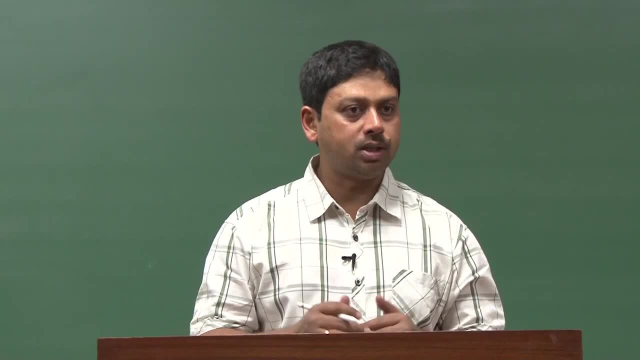 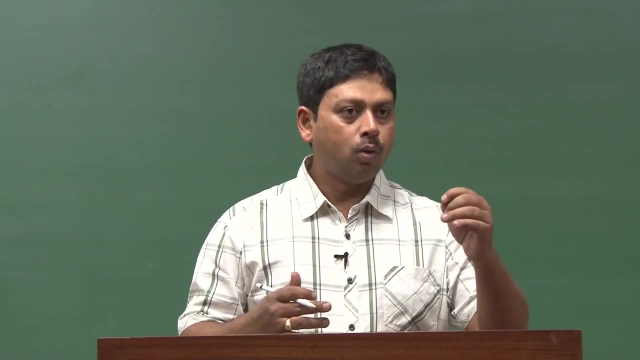 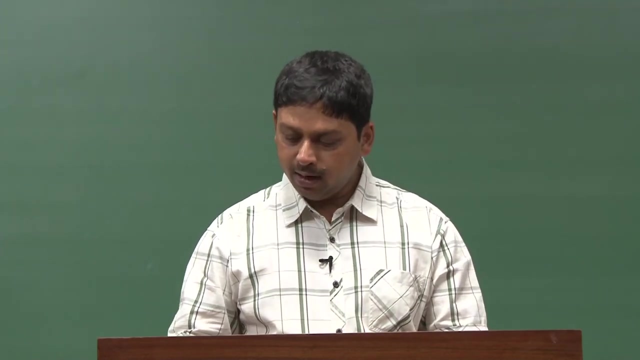 at triple point. That will give us a measure of the temperature That is in a gas thermometer. Similarly for other cases, for solids and other, you know, mercury, we calculate the property by looking at the changes in the volume or changes in the pressure and things like that. 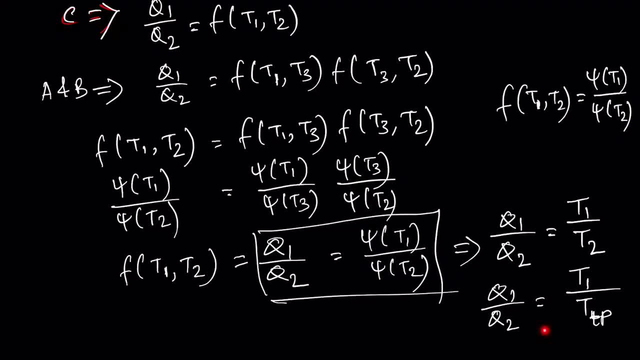 Here, thermodynamics temperature. we are calculating the temperature by calculating the heat input and output, And that is possible because Carnot engine gives us that. Remember that for ideal cases we exactly know that Q1 by Q2.. So in ideal cases we know that Q1 by Q2.. 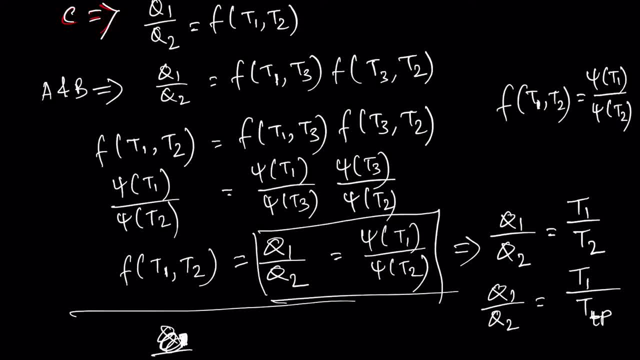 So in ideal cases we know that Q1 by Q2.. So in ideal cases we know that Q1 by Q2.. So in ideal gases case, we know that Q1 by Q2 is exactly as T1 by T2. That is from our normal temperature definition itself. it gives that in ideal gas. 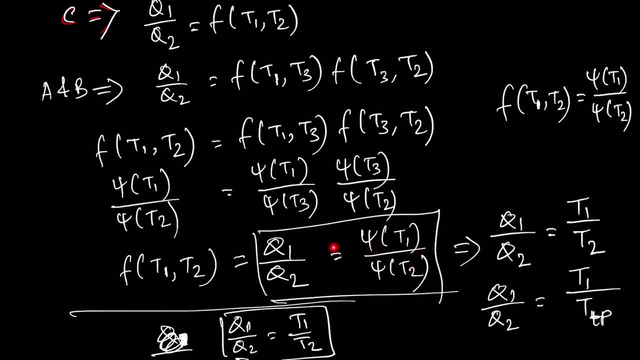 However, in general, for non-ideal gases also, we can write the ratios of heat input output as a function of the individual temperatures. Thus Kelvin actually decided. you know, given this Kelvin scale, And one can see that When one of that will go to 0, then let us say: you know, in order for the efficiency to 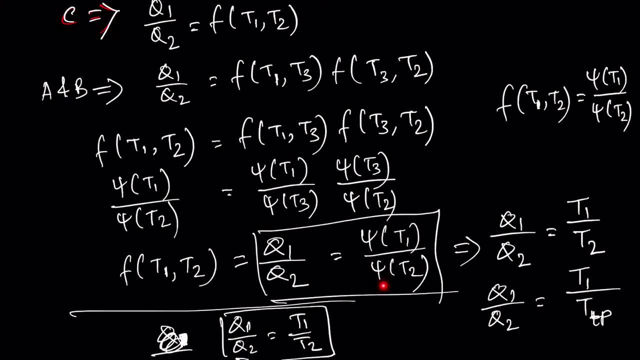 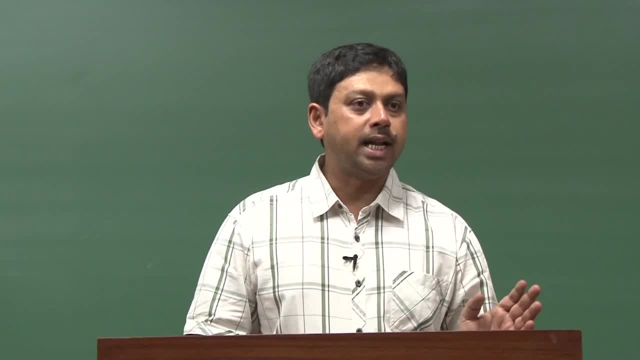 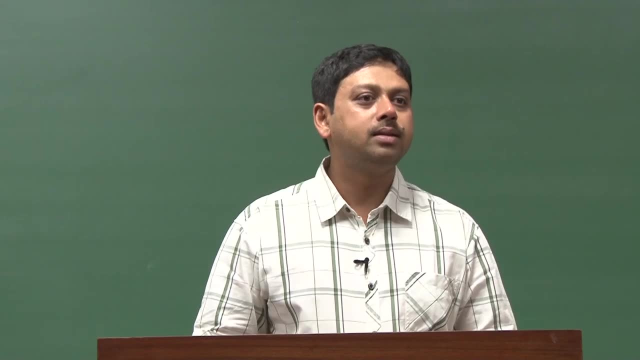 go to 1, the one of the temperature has to go to 0. And in that the heat output will be 0. There will be no heat going out, So it becomes an adiabatic step itself. So when the isothermal and adiabatic becomes equal, at that point your efficiency will become. 1, okay. 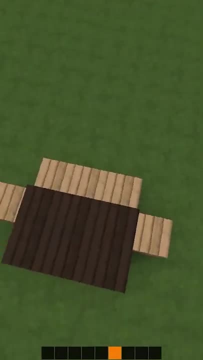 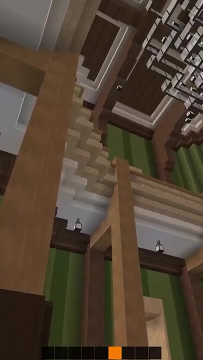 So I just finished building the world's smallest Minecraft house. It's super compact and I can fit everything I need inside of it. Let me show you the inside. Yeah, so basically it's not too bad. I tried to fit everything I needed inside of it. 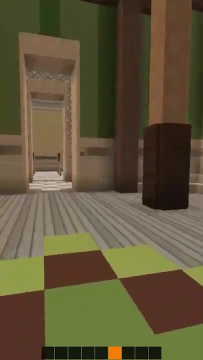 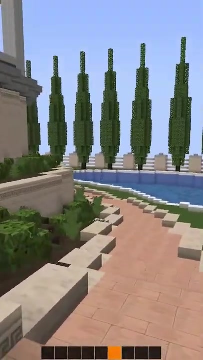 and I think I did a pretty good job. Yes, we have the main entrance here, and over here is the dining room and over here is the balcony and down here is the pool area. So, yeah, this house is pretty spacious for its size.